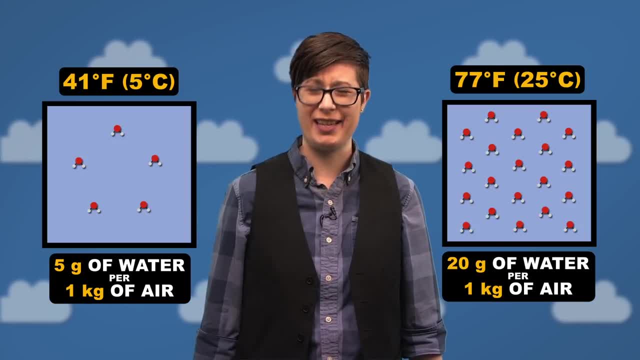 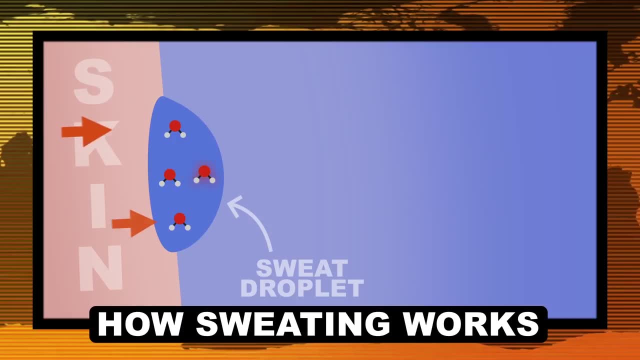 So why is it that the second example would feel so much more sticky? Because of how your body cools itself With sweat. Sweat cools your body down Because water molecules in it absorb thermal energy from your skin, evaporate and take. 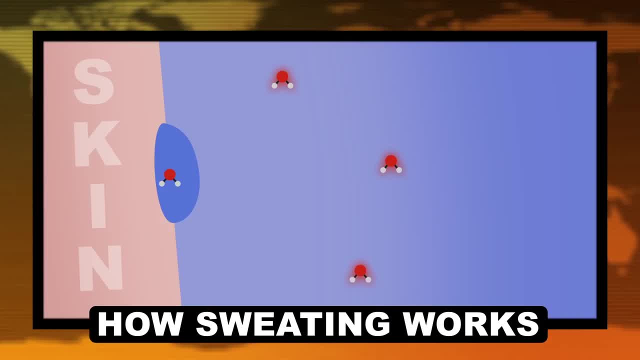 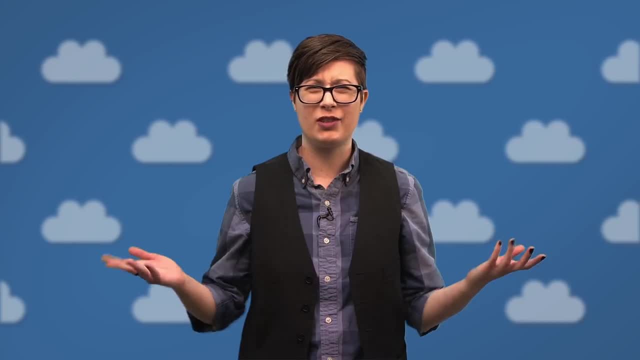 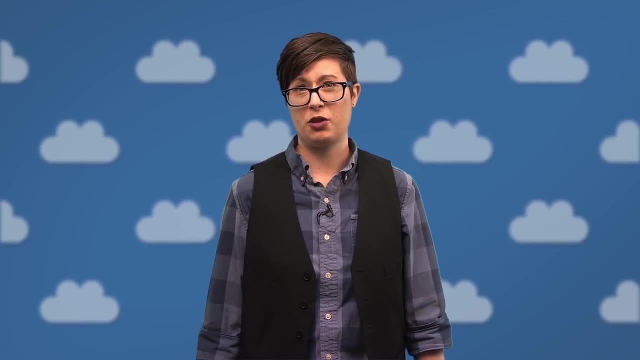 some of the heat energy with them. If the air is at 100% relative humidity, there's literally nowhere for that sweat to evaporate off to, So it stays stuck dripping down your lower back or in your armpits. At lower temperatures your body won't produce as much sweat, so it's less of a problem. 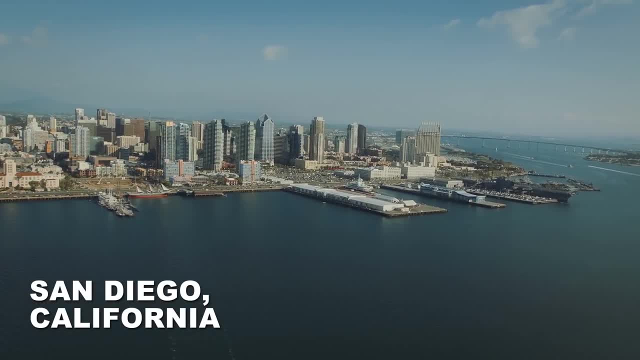 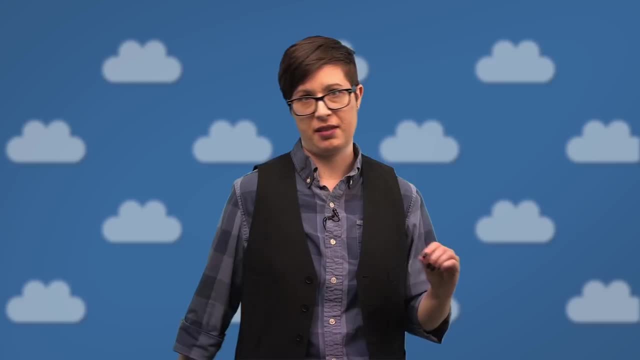 If you live in a place with consistent year-round temperatures, you can rely on relative humidity to inform your wardrobe choices. But anywhere else- and we cannot all be so blessed as to live in San Diego- it alone isn't going to give you the info you need to be prepared for the day. 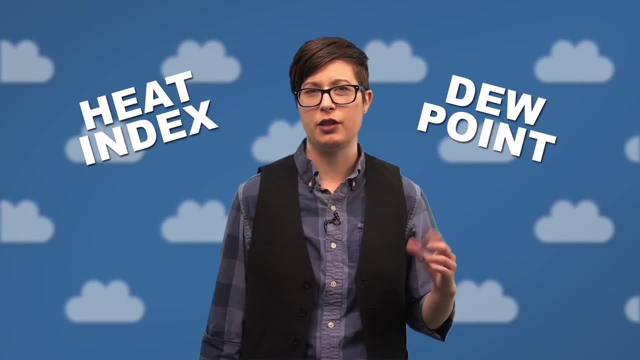 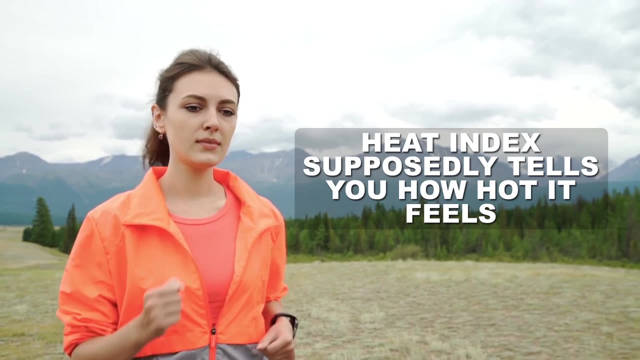 This is why meteorologists also use heat index and dewpoint to clue us in. Heat index supposedly tells you how hot it feels with any given temperature and humidity. So, for example, if it's 92 degrees Fahrenheit with a relative humidity of 85%, the heat index is. 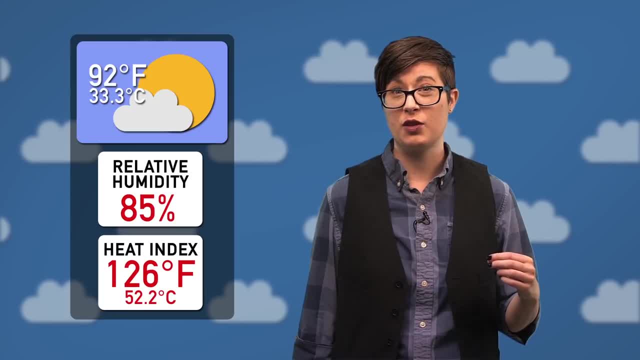 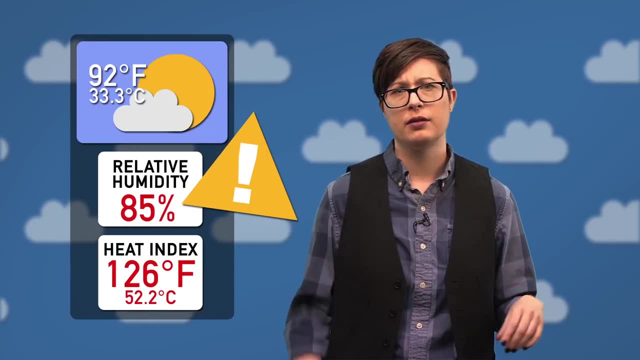 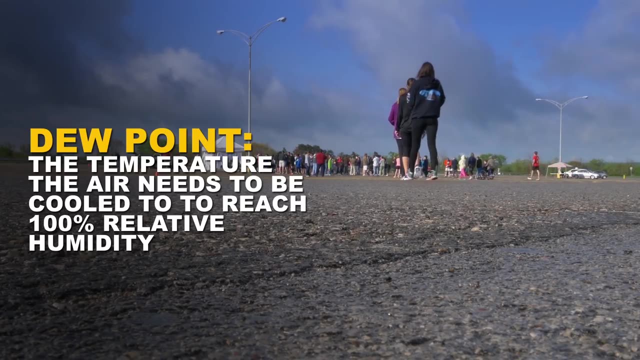 126 degrees Fahrenheit and the National Weather Service would tell you that heatstroke is likely, so stay inside. This can be useful, but how it feels is pretty subjective. Dewpoint, on the other hand, is objective. It's the temperature that the air needs to be cooled to to reach 100% relative humidity. 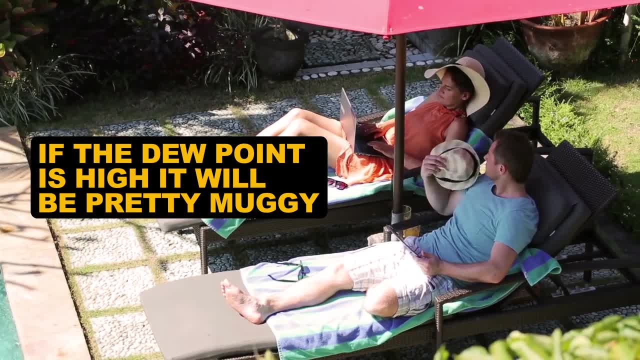 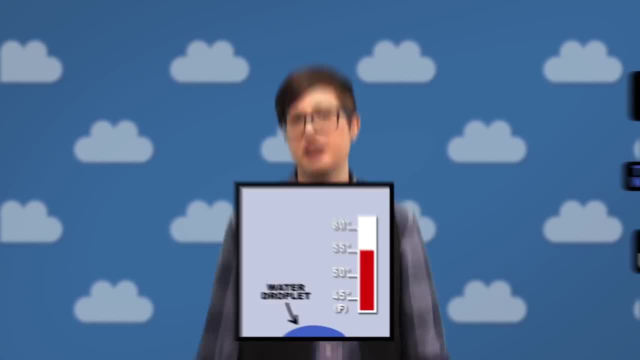 You can imagine that if the dewpoint is high it's going to be a pretty muggy day To understand how it works. take a look at this little box here. Let's say that inside the box it's 55 degrees Fahrenheit with a relative humidity. 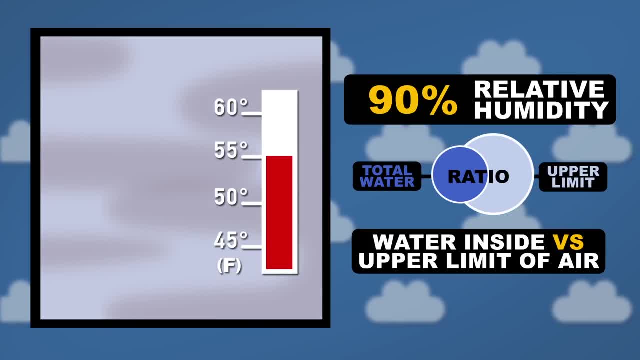 of 90%. At this temperature, the air is capable of having more water dissolved in it than is physically inside of the box. If we lower the temperature slightly to 52 degrees Fahrenheit, the upper limit of the air decreases slightly to an amount equal to that of the water trapped inside of the 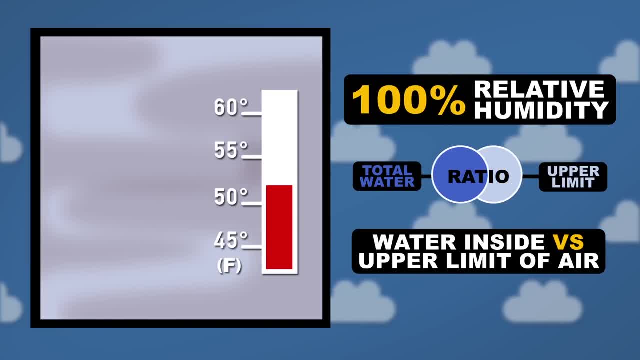 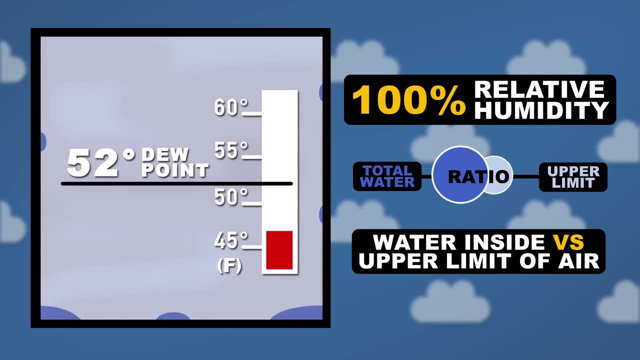 box. This means that we've reached 100% relative humidity. This 52 degree sweet spot represents the dewpoint. If you get colder than the dewpoint, the air would be unable to dissolve all the water and condensation or dew would begin forming inside.